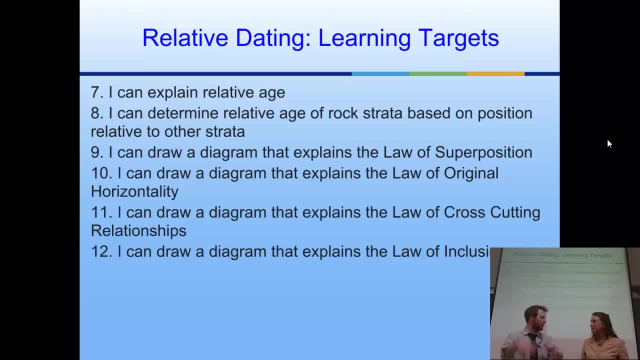 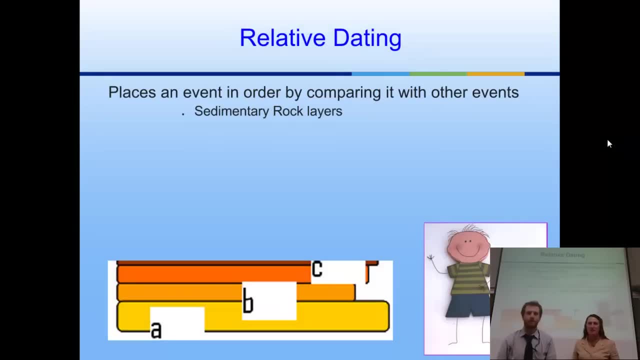 Yeah, They're going through some sort of crazy way to do it, but all at the same end point. Yeah, Cool, Sounds good. All right, And this is a slide deck that has some fill in the blank parts to it, So we'll be showing you what those correct answers are and make sure that you're recording those. 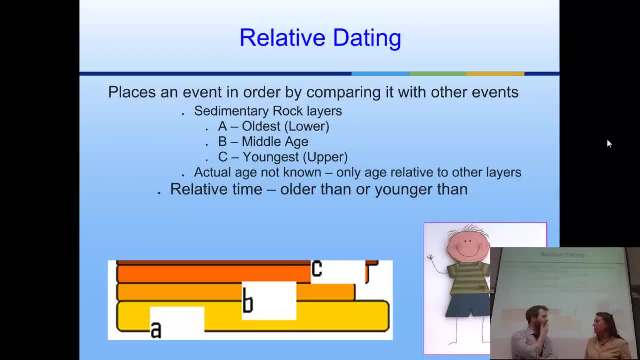 as you go through the slideshow in your packets. Yeah, Absolutely, They've got these pages in their packets this time, Great. So we're going to start out with A little relative dating. Good, Now, relative dating. it's actually pretty simple. 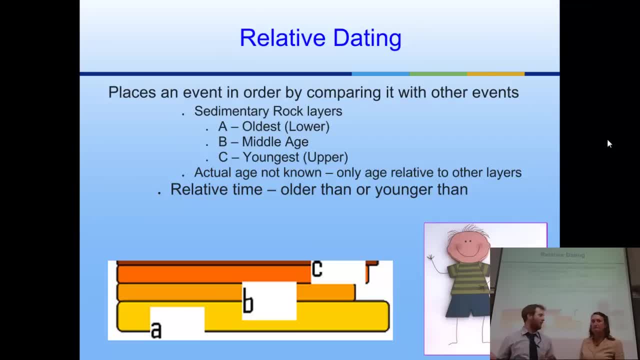 All you're doing is you're putting events in order, just on when they happen. We don't care about numbers whatsoever. Right? So I'm older than you are and you're younger than I am- Perfect, Just like in this picture of the two kids, the bigger kid is older than the younger kid. 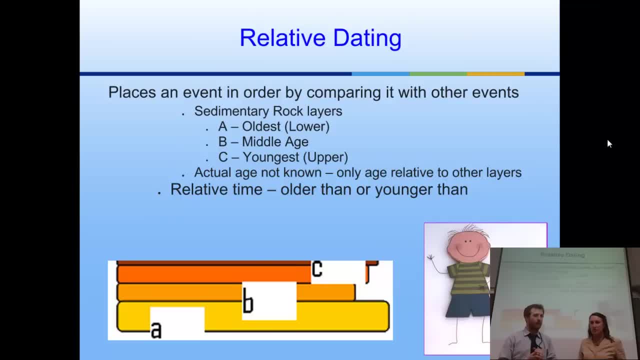 No idea the age of any of them, Okay, And so we've got a little picture here, a diagram here that shows an example of relative dating, the sedimentary rock layers, And what we can see is that the one labeled A, which is down here on the bottom, 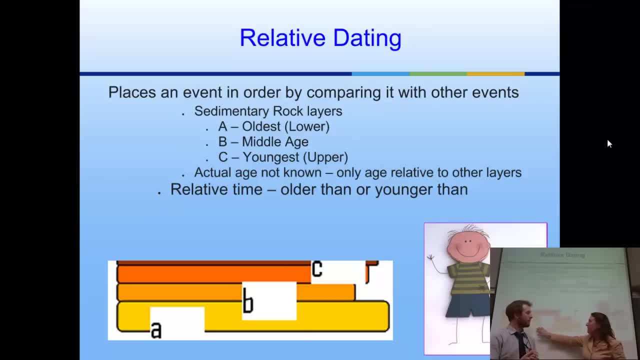 we know that that one is the old one, And then the B layer would be- It's right in the middle- A little bit younger, And the C layer on top is the youngest because it's sitting on top. And do we care about how old the rocks are at all? 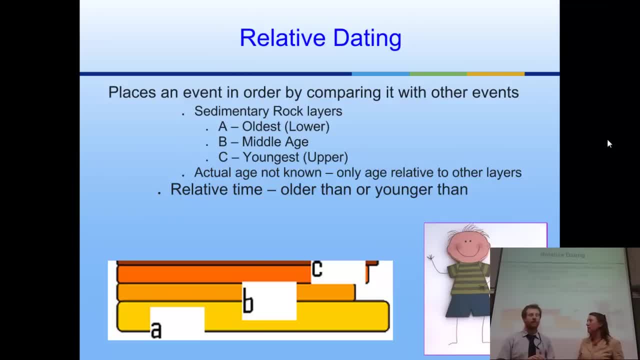 No, we don't. We only care about whether they're older than or younger than. We don't care about whether they're 10 years old and 12 years old. Perfect At this point. Okay, So let's talk about some of those. 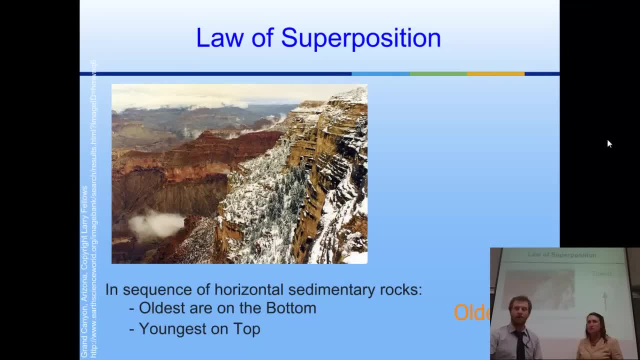 We have some really basic laws that we talk about, And the first law is the law of superposition, And it simply just states that the older rocks are on the bottom, younger rocks are on the top. Okay, It's as easy as that. 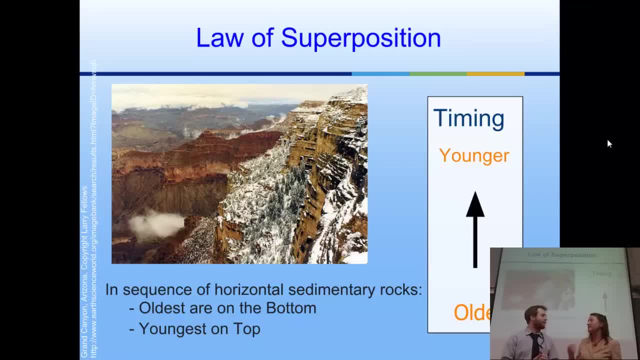 The important thing to remember here is that's in an undeformed sequence, where things haven't been flipped over, which we see sometimes, but not all the time. So a lot of times you just see a rock towards the bottom. If it hasn't been flipped, you know that one's the oldest. 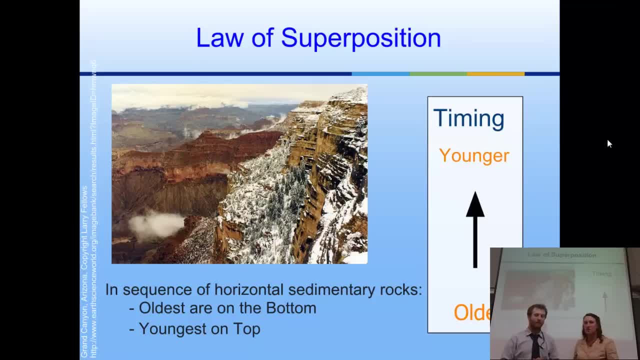 Rock on the top that one's the youngest. So if you're out in a beautiful place, like is shown in this picture, the Grand Canyon- you've got a nice sequence of sedimentary rock layers. You're looking down at the bottom of the canyon. 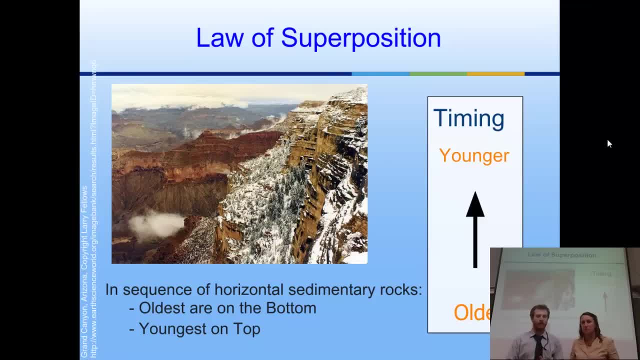 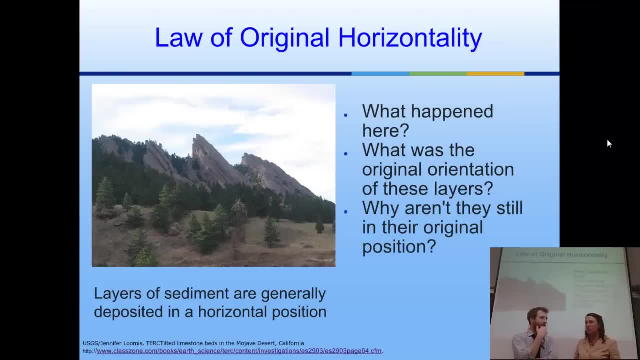 old ones there up at the top along the rims. young ones, Perfect, Easy enough. Good Law of original horizontality. I think that one says the whole thing Originally. all the rock layers, if they're sedimentary rock layers. 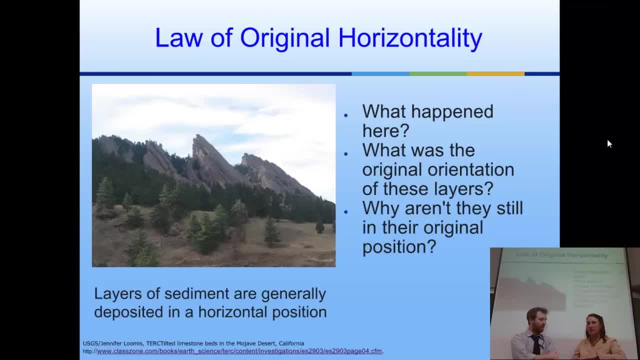 they were deposited horizontally flat, So not tilted, not standing up on end, not folded and not faulted, but just lying flat. Yeah. So if we were to look at this outcrop here and somebody asked what happened, I would say: well, you know. 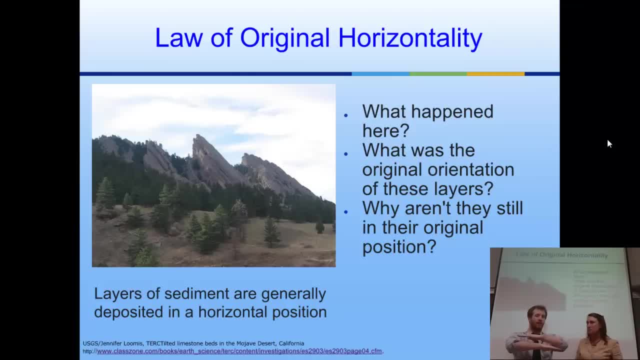 originally those rocks were probably laid down pretty flat, horizontal, So something must have happened to tip them up a little bit. So maybe some plate tectonics, a mountain building event, something pushed those rocks together to make it so they're not horizontal anymore. 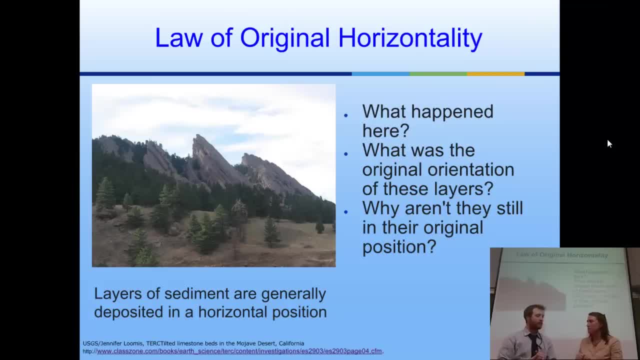 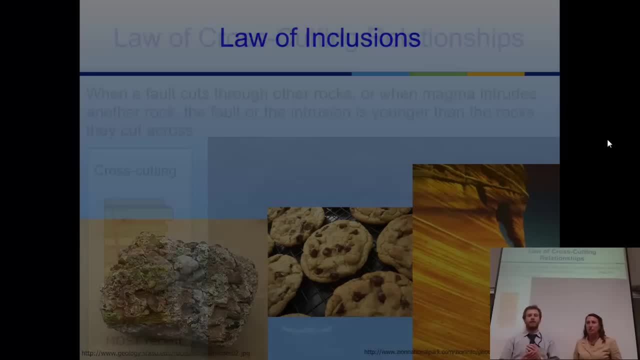 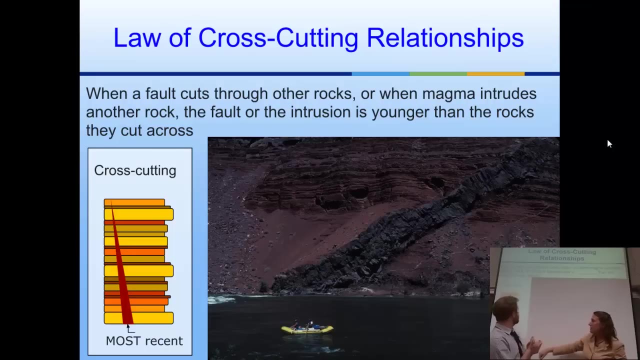 Pushed them together or pulled them apart and sheared them right- any of those things that we remember from structural geology? Okay, great. Next one: The law of cross-cutting relationships. So here we have a nice stack of rocks layers. 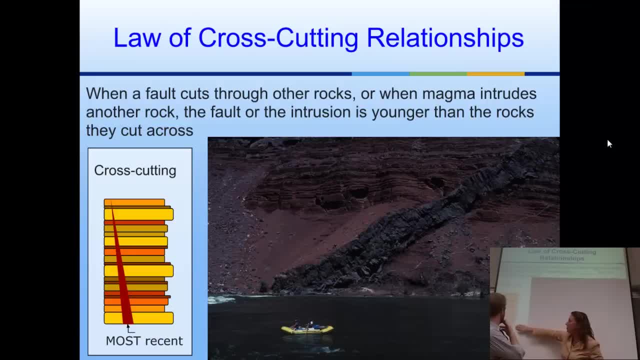 and you can see the oldest at the bottom, the youngest on the top. So this gold one at the very bottom, the orange, rusty color one at the very top, And then, cutting across all of them, is that arrow-shaped triangle, right Yeah? 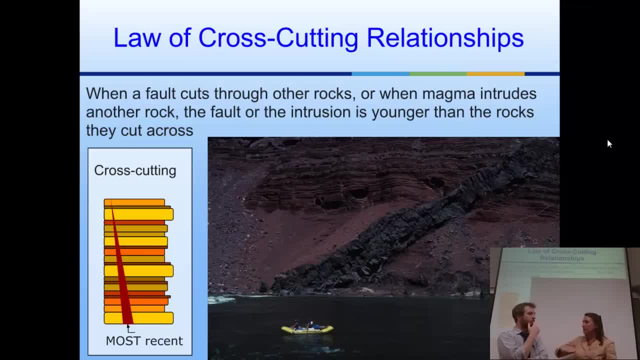 And we know for that arrow-shaped triangle to have cut across, those other layers had to already be stacked up there. Yeah, because we couldn't make that cross-cutting, we couldn't make that without the other layers being there, Right? A lot of times they say like when you rip a piece of paper. 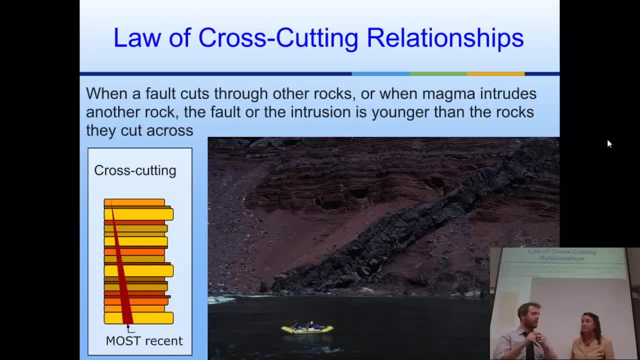 the rip is like that cross-cutting: the paper had to have been there first and then the rip, Yep. So what we need to fill in here? when the fault cuts through other rocks or when magma intrudes another rock, the fault of the intrusion is younger than the rocks they cut across. 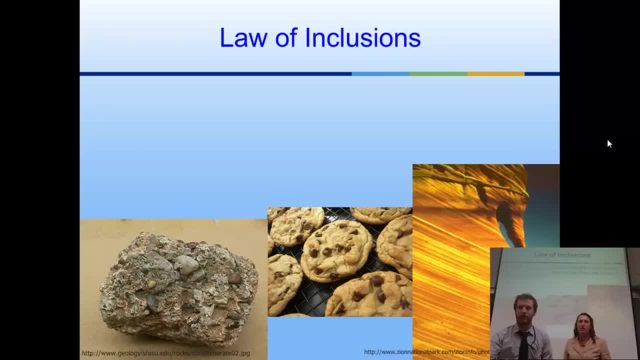 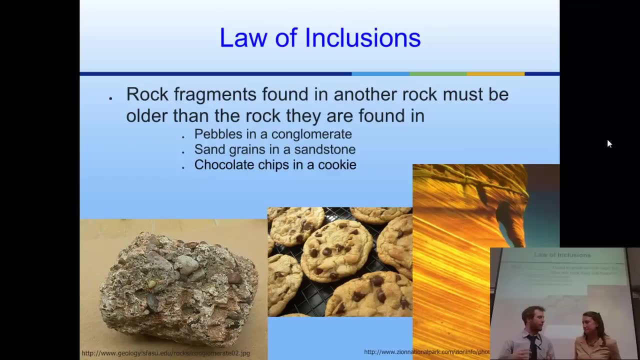 Perfect, easy enough, Great, Okay, let's go to the next one. We got the law of inclusion, okay. So basically, the law of inclusion just states that rock fragments that are found in another rock, the fragments have to be younger. 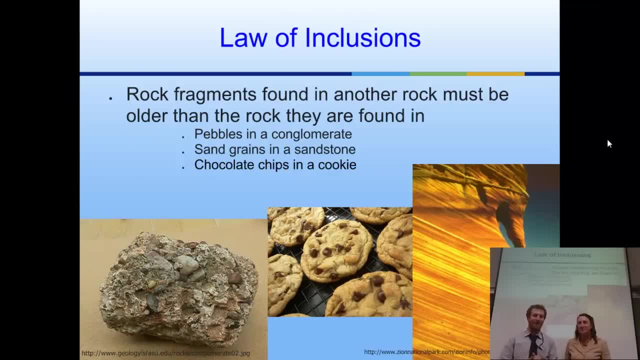 Sorry, older Fragments have to be older. Sorry, have to be older, older, older. Okay. so if we looked at the first picture, we've got a conglomerate Yep. It's got the rounded pebbles in it. 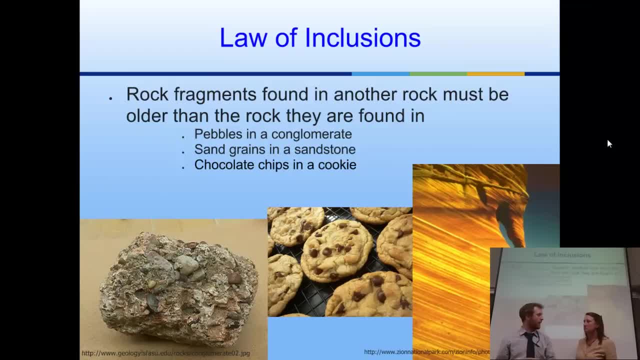 So the pebbles had to have been there first in order to make the rock Perfect. Okay. Same thing with our chocolate chip cookie. The chocolate chips were there before the cookie was there, so they're older than the actual cookie, Mm-hmm. 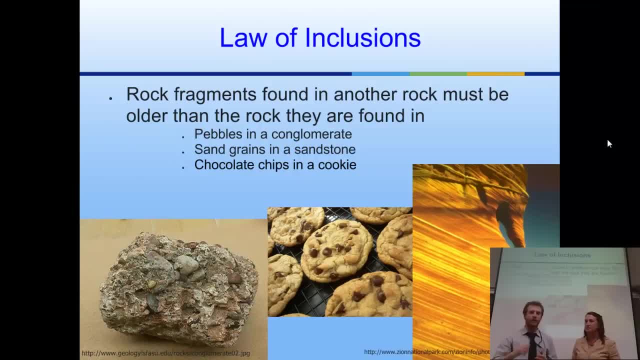 And then the last picture. all the way to the right, you can see it's a sandstone, so the sand grains had to have been there before you could have made the sandstone Mm-hmm, perfect. Sounds pretty straightforward and simple, right. 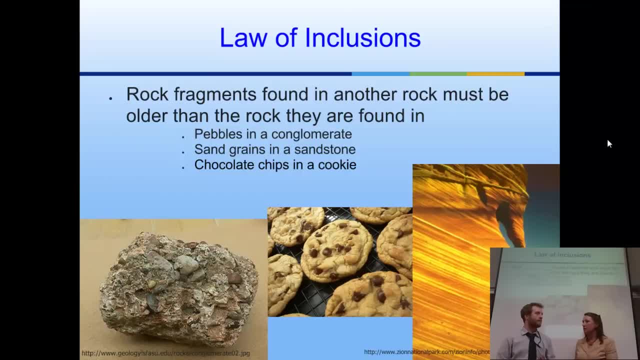 So we might find the law of inclusions when we apply that with some fossils that are found in a fossiliferous limestone. Mm-hmm, Anything that's included in another rock is older Cool Good, All right, so now we've got some more learning targets. 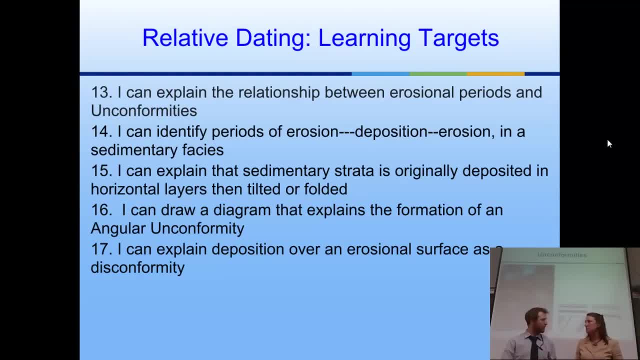 Take a pause on these, because we're talking about something similar, but a little different- A little bit different at the same time. So what we're going to do next is we're going to talk about how we take those laws and we apply them to unraveling the history of a sequence of rocks. 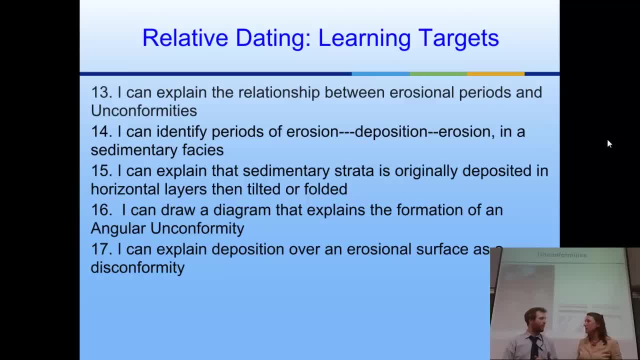 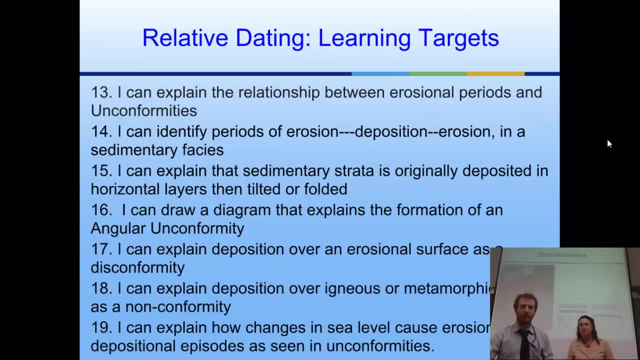 or an outcrop that we're out looking at. Okay, So you're going to be able to understand what happened, why it happened and in what order it happened. Perfect, Okay, Okay, so that brings us to something that we have here. 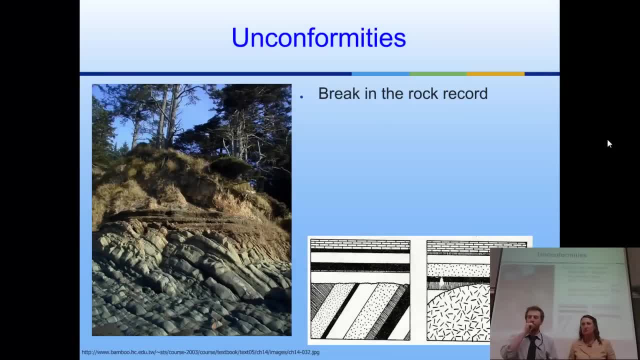 and it's called an unconformity. okay, So an unconformity, it's just a break in the rock record. okay, Before we saw all these nice little perfect stacks. but geology isn't perfect like that all the time, okay. 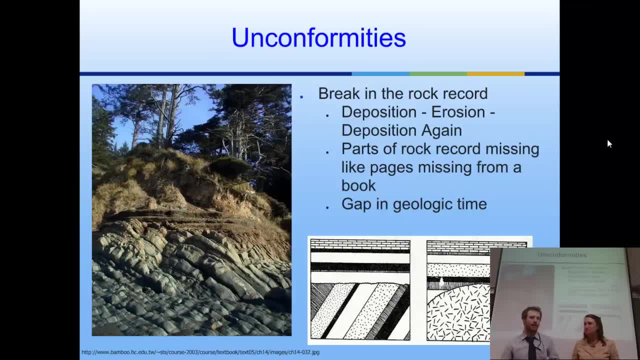 We end up changing some things around. So sometimes we're depositing rocks, sometimes we're eroding rocks, sometimes we're depositing them again. okay, And we're trying to tell the story based on some of the pictures that we see there. 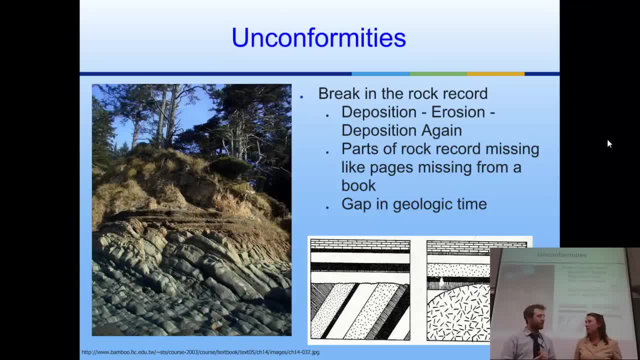 Okay. So what we see is we see parts of the rock record that are missing, like pages missing from a book, Okay, Okay. And we have to remember, as we go through talking about unconformities, that when rocks, when sedimentary rocks are being deposited, 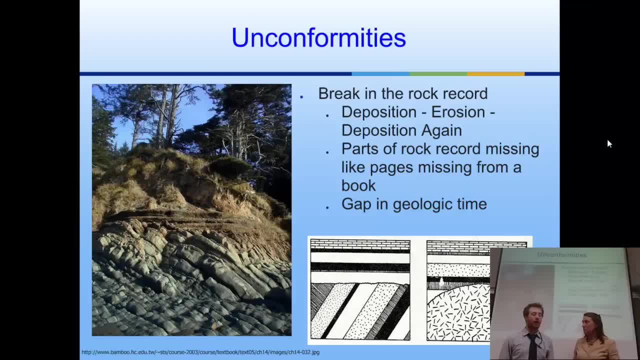 that most often happens underwater. Okay, So we're going to talk a little bit about sea level rising and sea level falling. When sea level is low, the rocks are exposed to the environment and they're being eroded away. When sea level is high, they're underwater. 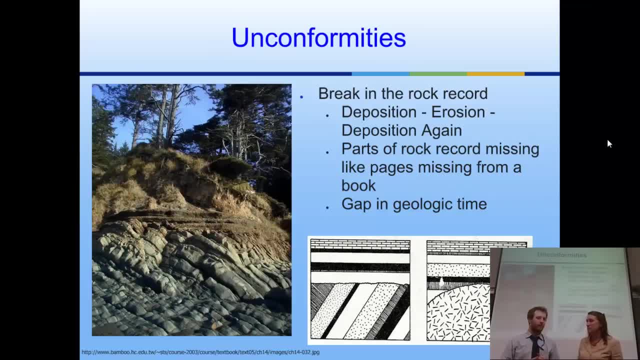 and rocks are probably being, or sediment's probably being, deposited and forms into sedimentary rocks. So we're going to interject some information here about sea level rising and sea level falling, as we're talking about erosional and depositional events. Okay, so when we say sea levels rise, it means we're depositing. 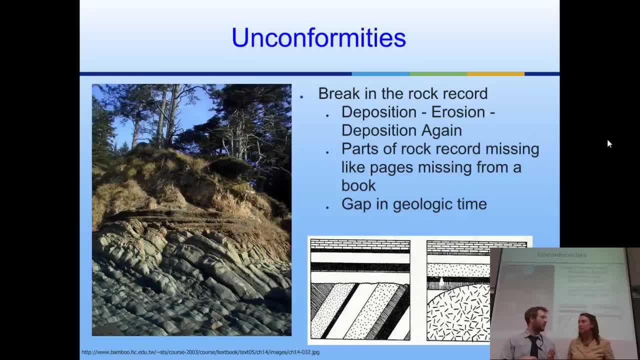 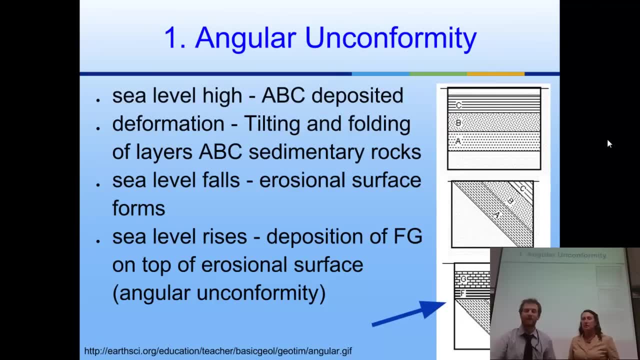 Sea levels falls. sea level fall were eroding. Yes, Cool, easy enough, Good, Okay so, oh Okay. so for the first type of unconformity, you guys got a lot of stuff to write for this one. 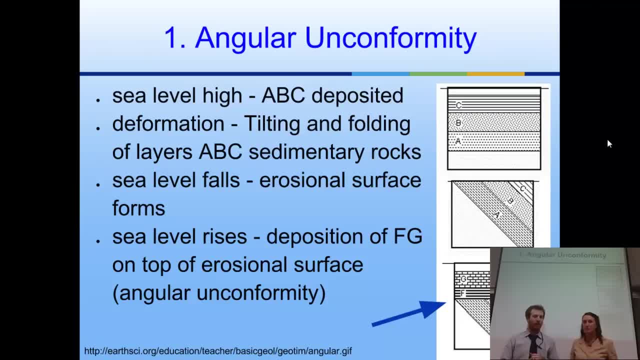 so we'll hopefully give you some time. If you need to pause, pause it, Yep, Okay. so first we're looking at a quick story that we have. So if we look at rock layers A, B and C- I know that A was deposited first- 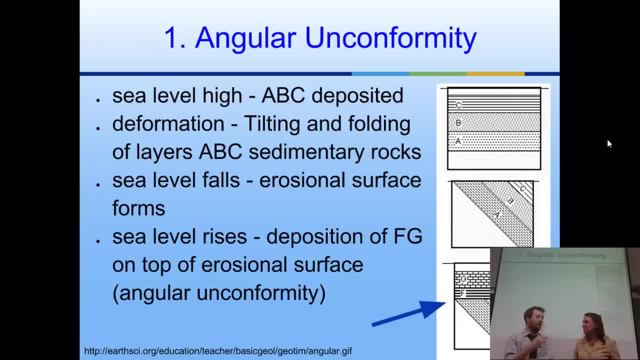 It's on the bottom Right, Then B, then C Right. The sea level must have been higher because I'm depositing rocks. Correct, Okay, something changed then. Okay, then I had some deformation, So I tilted my rocks because I can see that they're on an angle. 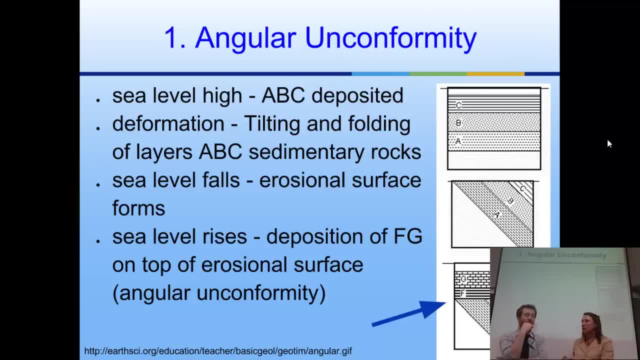 Mm-hmm. Okay, So let's go back just one second. Oh sorry, yeah, And the first one. when A, B and C are deposited, we're going to use the law of original horizontality to show that they were deposited flat. 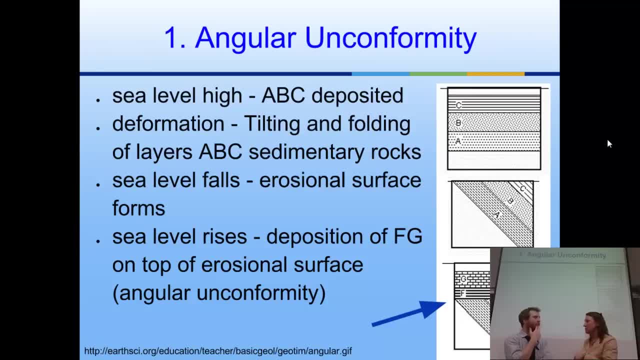 Okay, When that sea level was high, right, Mm-hmm. So now we're seeing the deformation, Gotcha? Okay, Good, Okay, so we deposited them, We had them flat, Then we tilted them, Then we got them angled a little bit. 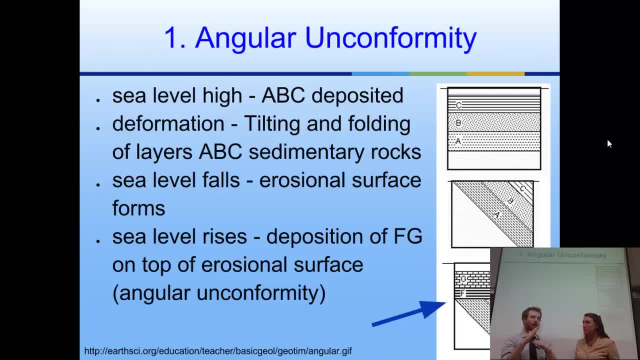 And then we have our sea level drop Mm-hmm. And we said, when sea level drops, erosion takes place. Right, So I start eroding part of my A, B and C searches, Yeah, Okay, Then my last one. what ends up happening is sea level rises again. 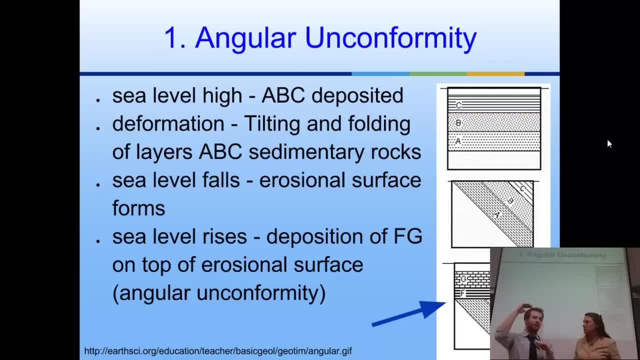 Yep, So all the way at the bottom, my sea level rises and I deposit layers F and G. Yeah, And I know, because of superposition, F is going to be older than G, Right And G is on top, so G is going to be the youngest. 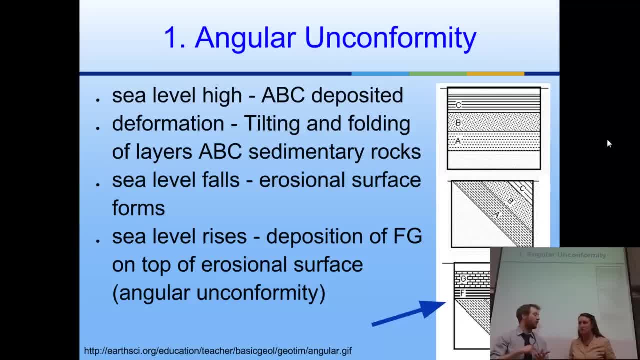 But we know F and G are also older, sorry, younger than A, B and C, right? Yeah, Yep, Like what's going on. Yeah, Okay, Okay, Okay, Oh, my goodness, Okay, Okay. 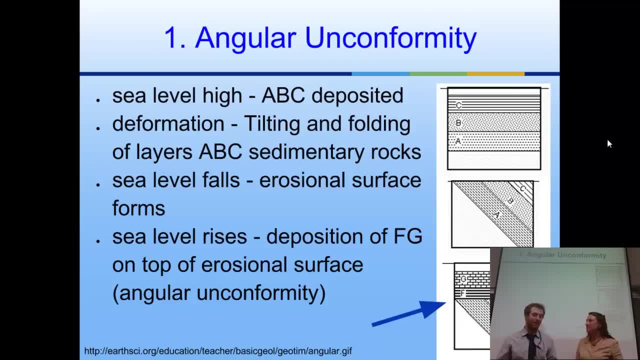 And this creates one of our unconformities, a gap in time where we have erosion taking place, because we've got that angular unconformity, I've got sharp angles underneath and then horizontal intersecting with those angles. Okay, So angular unconformity- that's this one- is usually the easiest to see, because you're 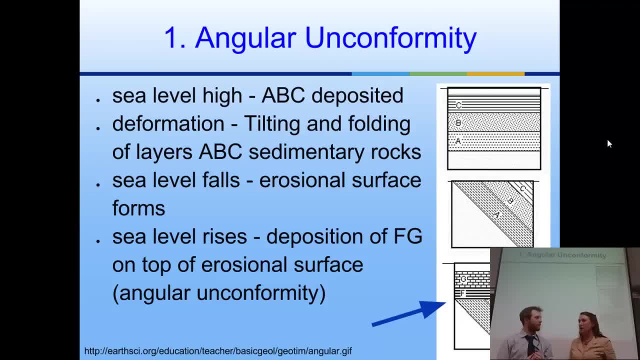 seeing the angle in between the layers. Yeah, And the unconformity itself is the erosional surface that sits below layer F in this case. Mm-hmm, Right, So it's the erosional surface separating F from A, B and C. 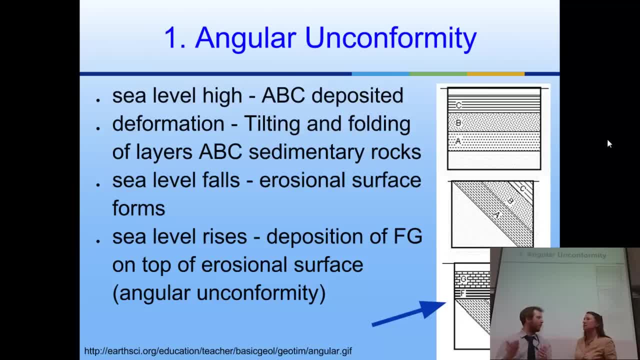 Okay, That's the actual unconformity, right, Because that's a gap in time. We're missing part of the story there. Yeah, And we have no idea what happened, Right, We can't figure it out, And it could be. millions of years are missing. 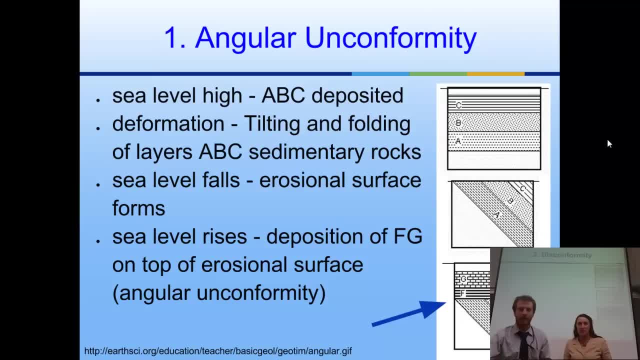 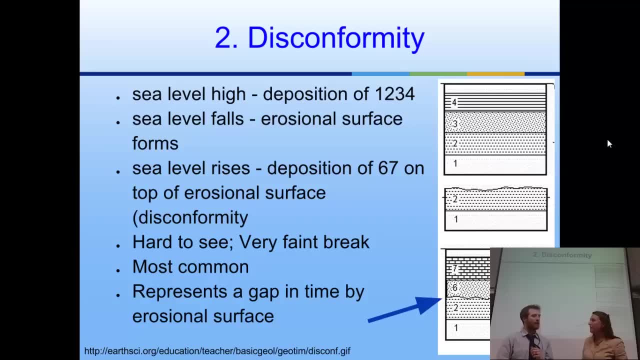 Oh yeah, All right, Good, Let's take another one, Okay, Second type of unconformity we see it's actually called the disconformity. This one's actually the most common one that we see, but it's the most difficult one to. 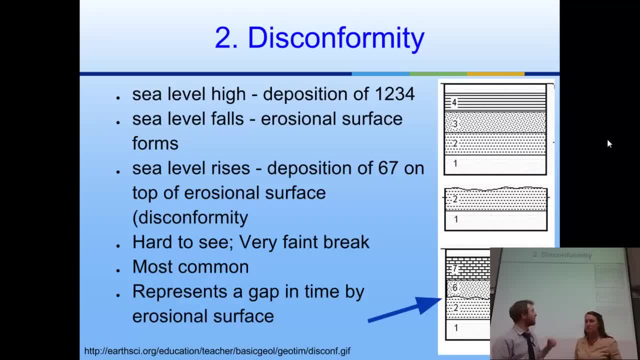 tell It is: yeah, So we've got the top layers that we're forming first. So we've got one, two, three and four And then originally horizontal superposition, oldest on bottom, youngest on top, And again those are deposited when sea level is high. 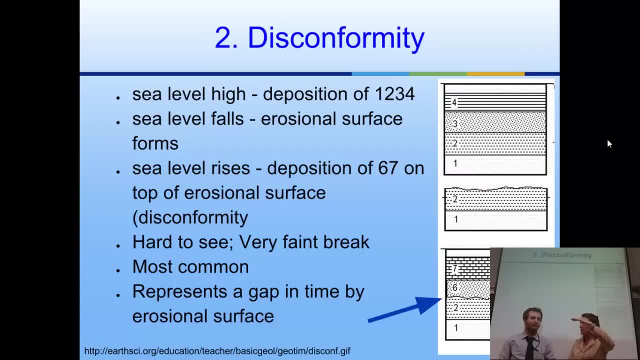 Mm-hmm, So we're getting a lot of deposition. Okay, So then sea level is going to drop Mm-hmm. We don't know how much it drops. What we do know is that an erosional surface formed there, completely eroded away layer. 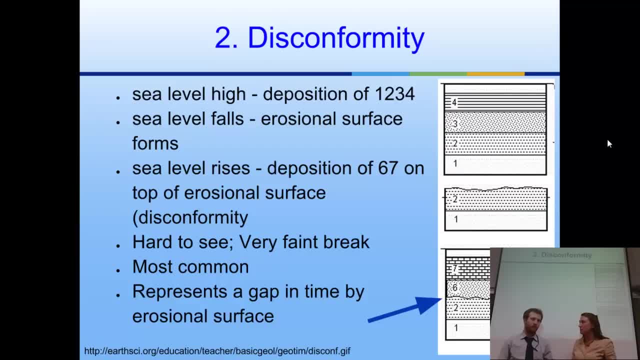 four, completely eroded away layer three and cut into layer two. Okay, So there's no evidence of layers three and four at this outcrop any longer, Totally wiped out. Now we've got the erosional surface that's going to be our unconformity on top of layer. 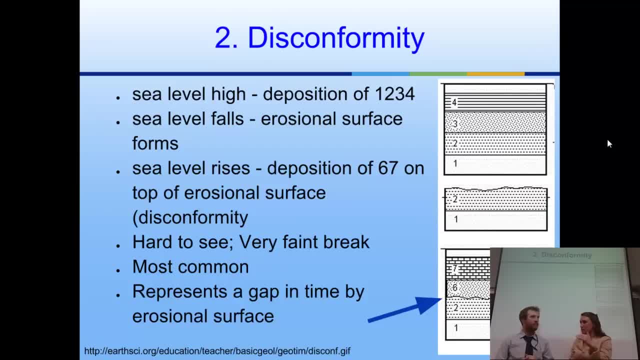 two, Okay, All right. So then, if sea level rises again after some time and new rocks are deposited, we've got layer six and seven deposited on top of one and two. Oh, okay. So now here's our unconformity, the erosional surface, that disconformity. 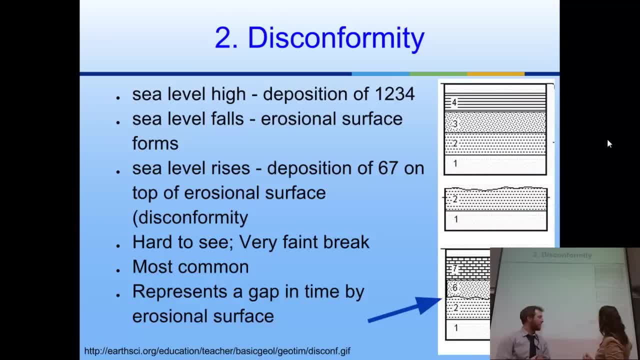 Okay, How do we know that? Yeah, How do we know that two and six aren't conformable? Oh my gosh, What clues are there? So we might have to find other outcrops where we would see like one, two, three and four. 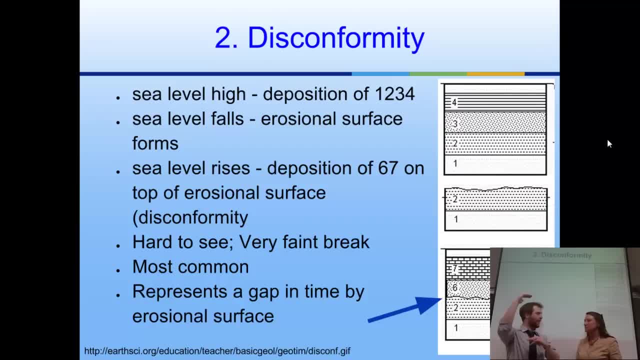 Mm-hmm. And then at our outcrop we see one, two, six, seven, Okay, Like what happened to those other layers, Yeah, And we're going to see a great example of that in lab, right, Yeah. 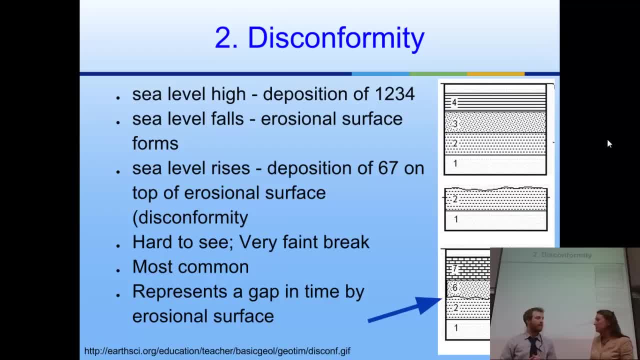 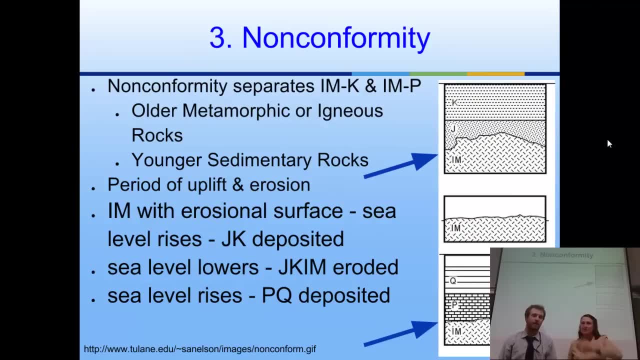 Absolutely Okay. Good, We might look at fossil data. Mm-hmm. All right, So there are other things that we can use to clue us in on that. Okay, All right, Good, Okay, So this one is a little bit of unconformity. 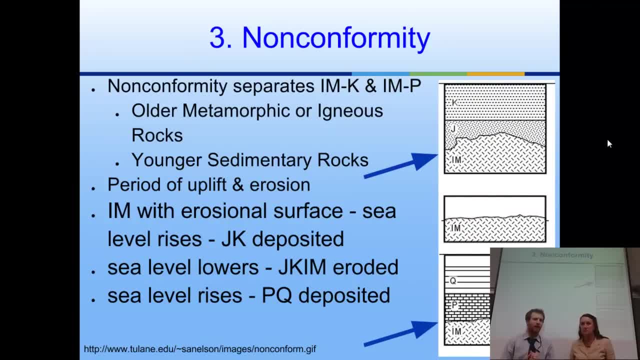 It's a nonconformity, Mm-hmm. Okay, This one a little bit easier to tell here. Okay. So basically what it does is it separates an older metamorphic or igneous rock from a younger sedimentary rock at some point. 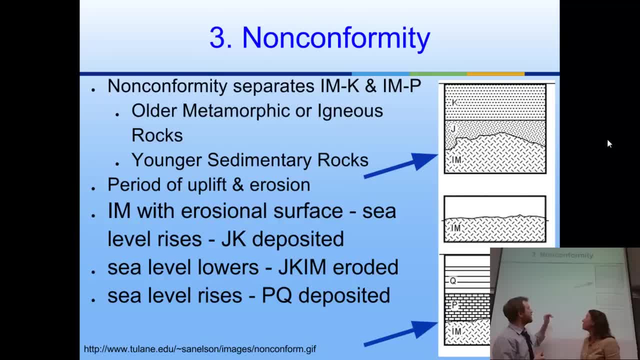 Okay, Okay. So if we take a look at the first one, we've got J and K and then IM. IM is just igneous or metamorphic Mm-hmm. So J and K had to have been there first for IM to be placed there, because it's igneous. 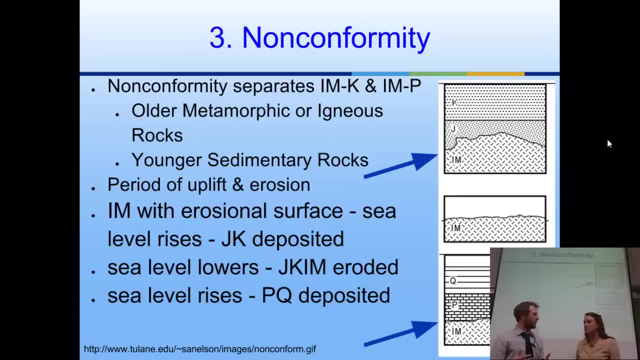 It cuts across it Mm-hmm. So that's our law of cross-cutting relationships. So I know that J is the oldest, then K, then M, I and M came Okay, Okay. So there's actually an alternate way to think about this one. 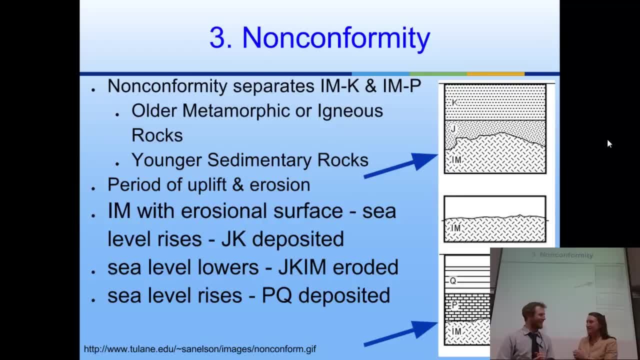 Oh my gosh, Let's see yours. Yeah, So it's possible that IM was there first. Oh, okay, That there was a lava flow, Oh okay, That was there and it was being eroded, and then maybe sea level rose and deposited J. 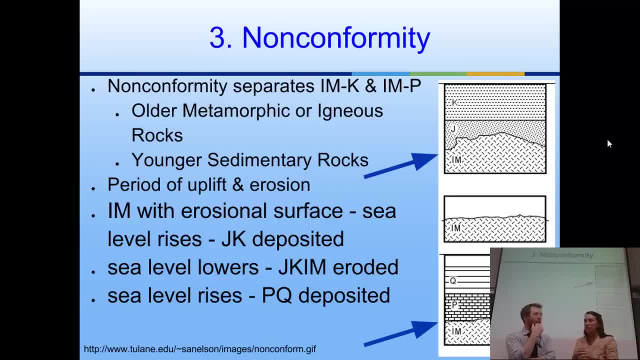 and K on top of IM? Oh, on top of it. Okay, So one of the things we're going to start to encourage you guys to look for is we're going to look for something called a baked zone, where, if J and K were there and then 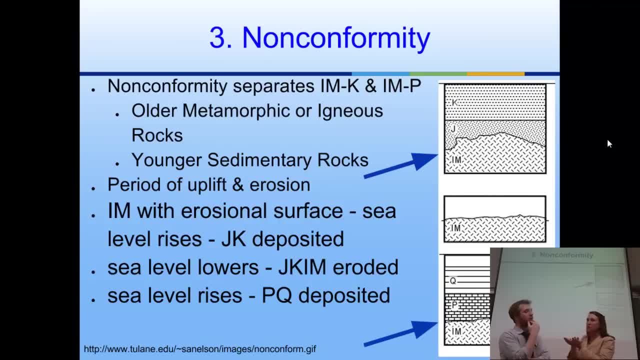 IM was intruded into it. it would actually bake layer J, Just like if your hand was there and I put a flame under it, it would burn your hand. Yeah, it wouldn't feel good If J was there and IM was intruded into it. it would burn that layer and you'd see evidence. 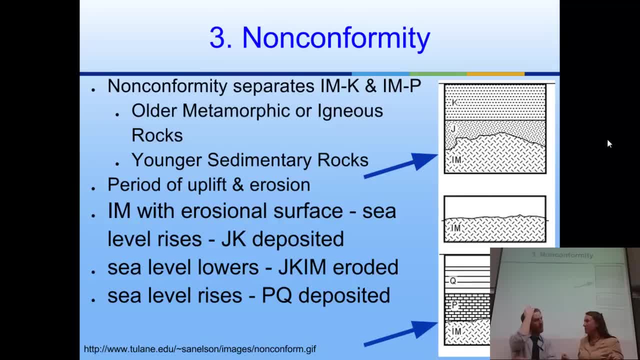 of-. Yeah, a zone around IM that was baked. Okay, So we'll talk about that more as we're going through the problem set. Okay, But realize with this you've got one little twist that you need to look for. 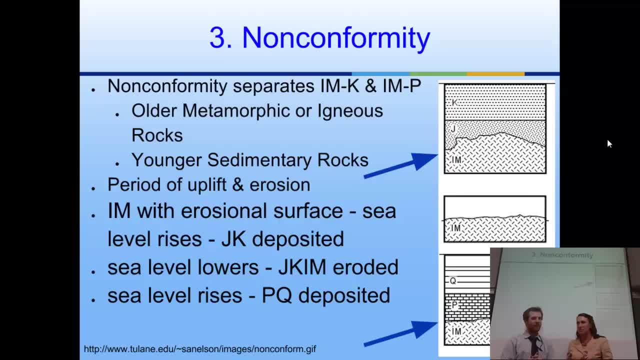 You need to look for that baked zone. Okay, All right. All right, So we end up having that igneous and metamorphic surface Right, And then we had J and K, whichever one ended up happening first. Yeah, If it's the baked zone, then we know that IM came later. 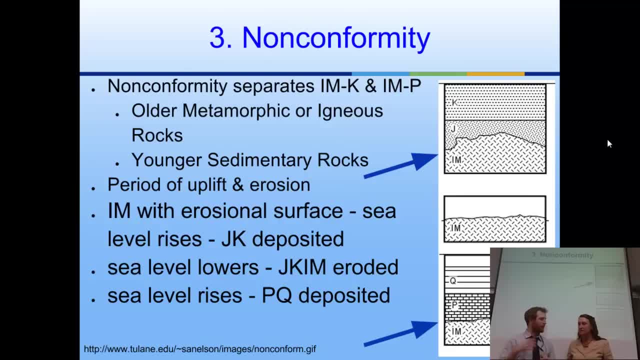 Right, Okay. Then we had sea levels fall and they eroded away J and K, And then we had deposition here of P and Q- Yeah, Okay, And then we had J and K. Yeah, And then we had J and K.